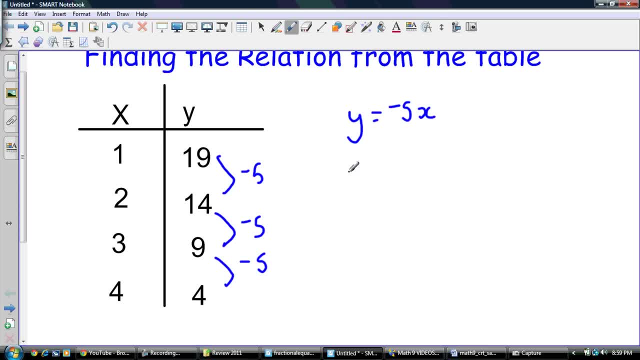 Now, that's not our relation for this table, because look, if x is 1, we get negative 5.. Negative 5 times 1, well, that's not equal to that's equal to negative 5, but I need 19.. 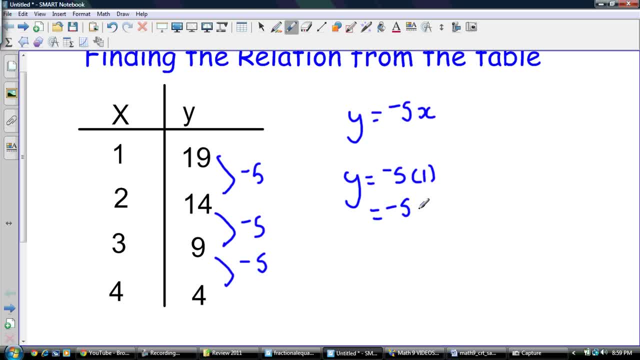 So how do I get, uh 19 out of that? Well, the way I get 19 is if I add 24, okay, So I get negative 5 times 1 is negative 5. Negative 5 plus 24 is going to be equal to 19.. 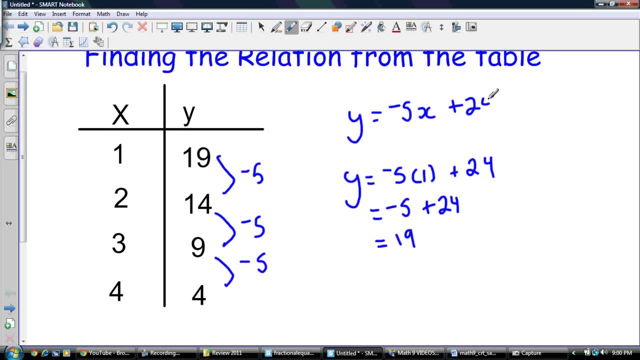 So my relation here is negative 5x plus 24, and that's equal to y. That's my relation for that table. And again, you can test another point 2 times: 5, negative 10, plus 24 is 14, okay. 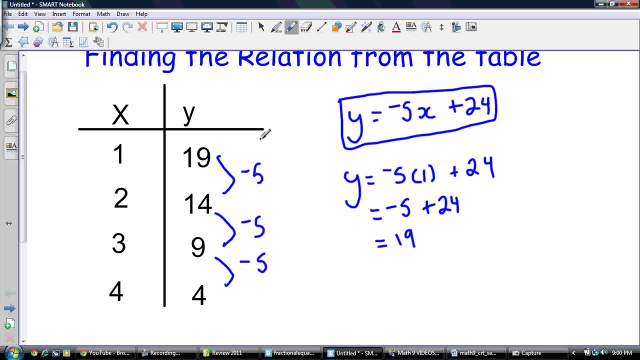 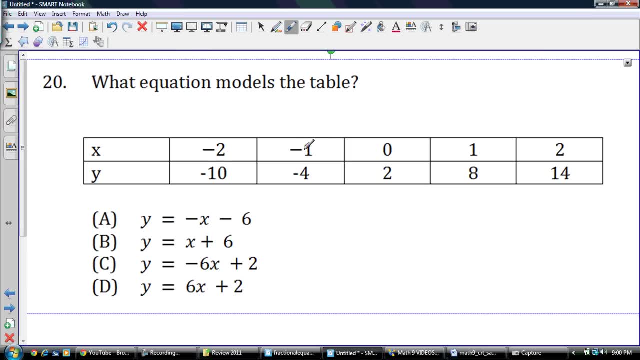 So you can test them, see if they work, and then you're in business. All right, let's try another one. This is a linear relation. This one's actually off your um practice. uh, final that I made up of. uh, comprehensive final I made up. 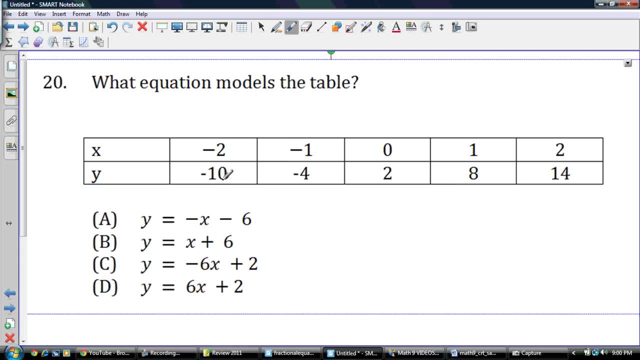 So this is a multiple choice question. So we're looking at what equation models the table. So we got my x's going on here. They're going up by 1, so we're good, And we have my y's here. 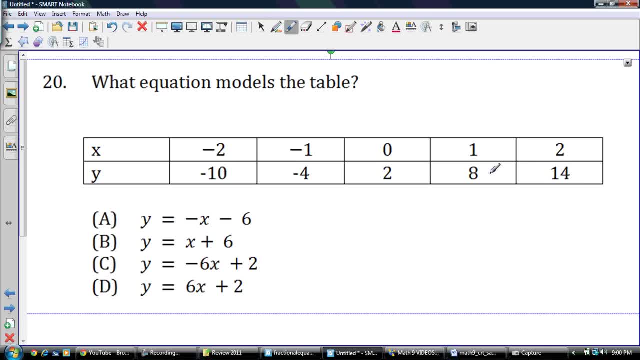 They are going down by 6, okay, So subtract 6.. Actually, they're going up by 6,, sorry So 6.. Going up by 6, going up by 6, it's going up by 6.. 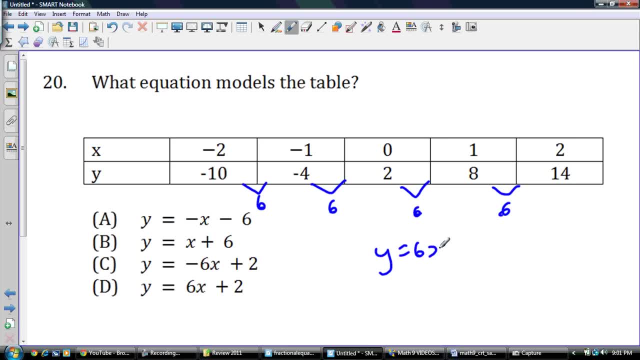 So we start off with: y is equal to 6x. So if you were on the test now, you could go bada-bing, bada-boom, shade in your bubble sheet. done deal, move on. But we'll find the plus 2 part as well. 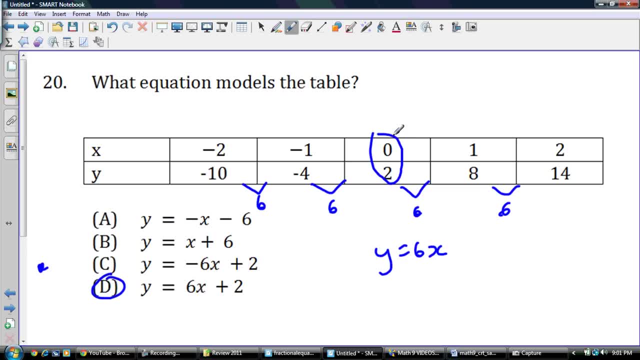 Now we have a special point here. We have 0, 2.. Anytime you have 0 for x, you always know that you're going to have to add that 2 there, right? Because 6 times 0, well, that's just 0. 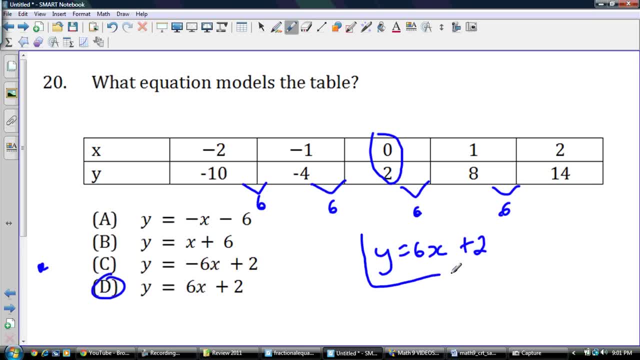 So in order to get 2, you got to add 2.. So that gives me my equation okay. So, guys, I hope that that's clear on how to find the relation from a table. It's an important skill. 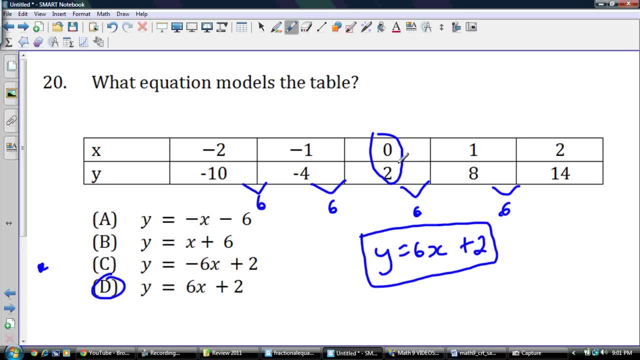 It's a fundamental to understanding the stuff that's in Unit 4.. Hope that helps. 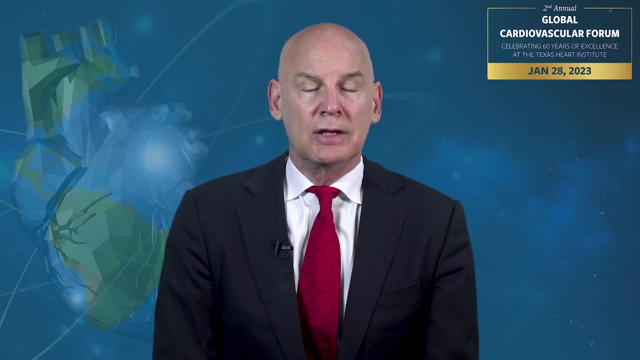 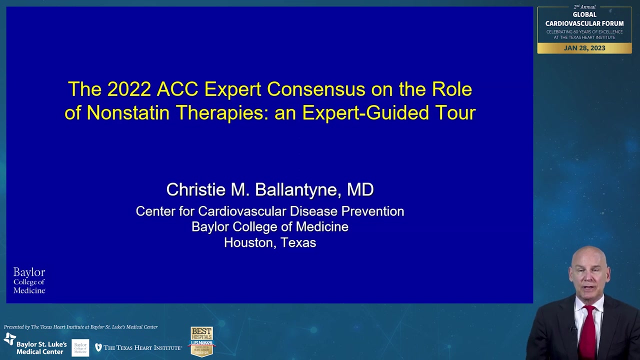 Hello, I'm Christy Ballantyne. I'm the director of the Center for Cardiovascular Disease Prevention in the section of cardiovascular research at Baylor College of Medicine And I'm going to discuss 2022 ACC: expert consensus on the role of non-statin therapies: an expert guided. 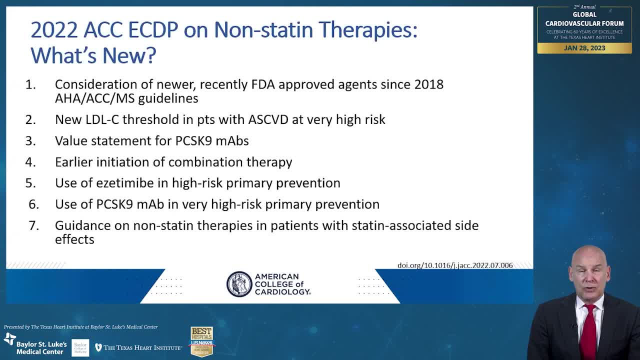 tour. These are my disclosures. Well, I was fortunate to be a co-author on part of this pathway. And what's new in here? Well, we consider the newer recently FDA-approved agents that have come out. There's a new LDL cholesterol threshold in the very high-risk. 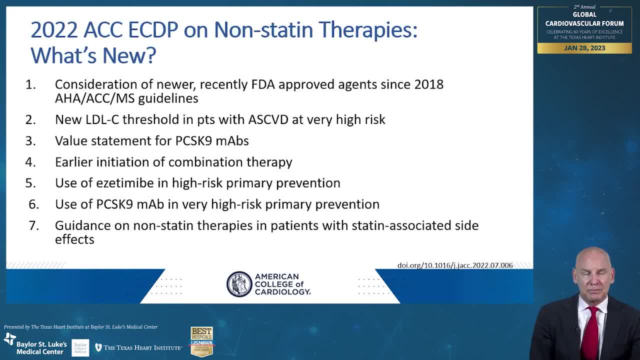 patients. There's a change in terms of the value statement on PCSK9 monoclonals and more focus on combination therapy. When do you use ezetimibe? When do you use PCS- monoclonal antibodies in very high-risk primary prevention And some discussion on non-statin therapies. 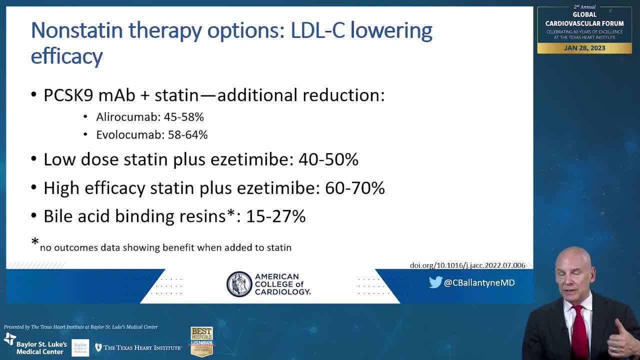 So non-statin therapies? Well, what are these? We've got the PCSK monoclonals. We've got ezetimibe. Those are very effective when you combine with statins. We've still got an old therapy of bile acid. 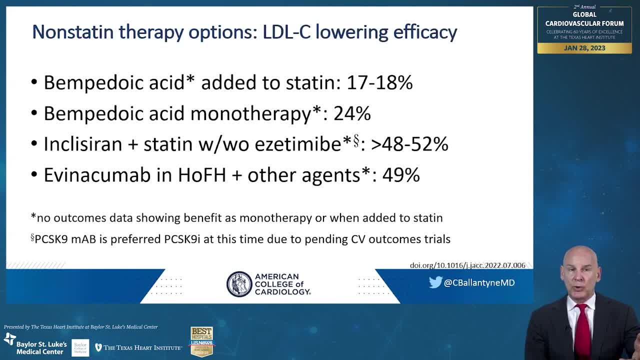 binding resins And we have some new therapies. We've got benpidoic acid. when you add it to statin, around 70% to 18%. It's monotherapy, It's about 24% And it also comes in a combination. 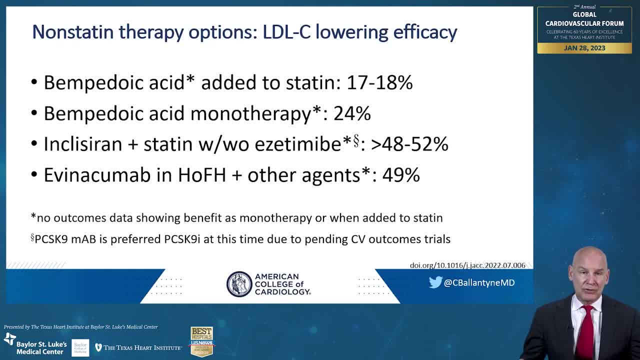 pill. We have Inclisirim. It's a very unusual agent, very long-acting, Once you're doing it chronically every six months. And we have Ebonacumab, which is a special consideration in homozygous FH People without. 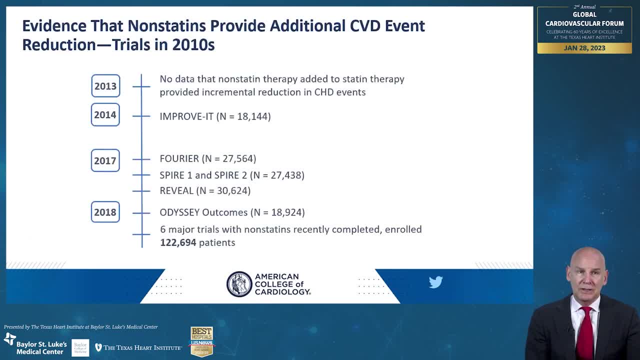 LDL receptors still lowers LDL almost 50%. So why are we having more change in our guidelines? Well, we have new data And there's lots of evidence for the benefits of non-statin therapies. These have been coming out since 2013,, but we have a large number of patients- over 120,000.